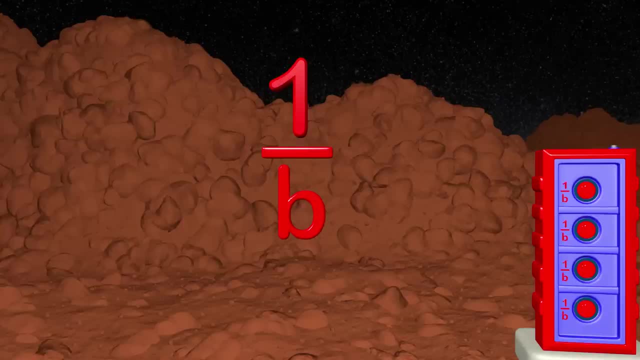 The letter b can represent any number. All this is saying is 1 over any number represented by the letter b. So it could be 1 over 2, 1 over 3, 1 over 4.. Well, you get the idea. 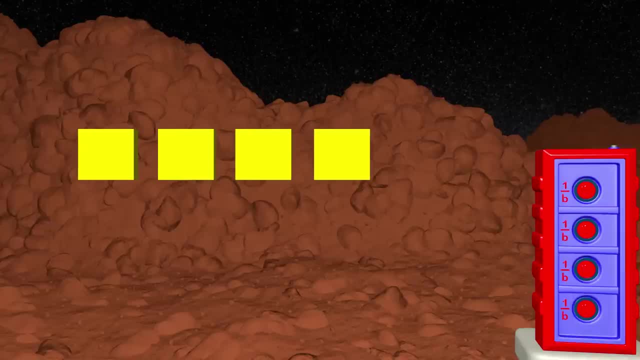 Here is a rectangle that is divided into 4 parts. Can you tell me what the fraction is for just this part here? This is 1 over 4, or 1 fourth. We can see that each of these parts is 1 fourth of the entire rectangle. 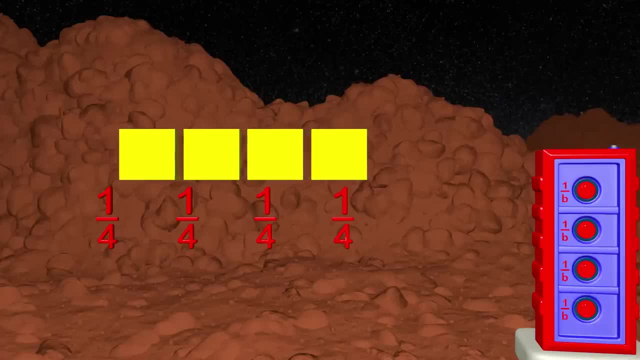 When you put it all together they make one whole rectangle. The battery only gets charged when taking one part of the whole, or in this case, 1. fourth, Let's get another fraction. Here is a rectangle with 5 equal parts. 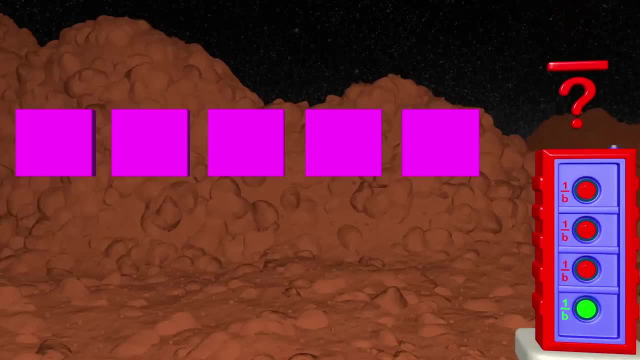 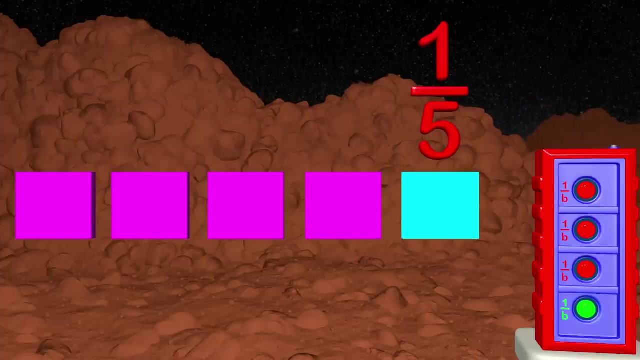 To write the fraction. let's start with the denominator. What number should the denominator be? The denominator is 5 because there are a total of 5 parts of the whole. All 5 pieces together make one whole. Remember that my batteries get charged with unit fractions which are just one part of the whole. 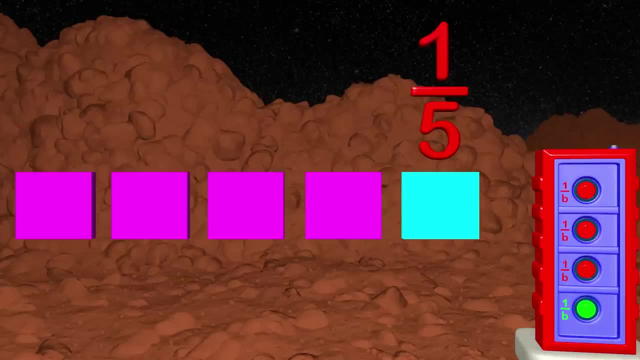 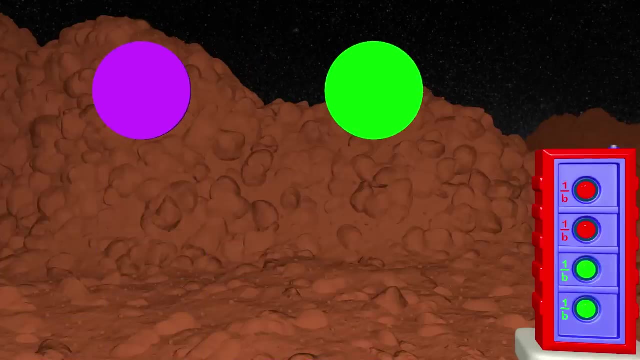 So we have 1 over 5, or 1 fifth. Let's put this fraction in the charger and try another one. Here we have two circles. Let's see how many parts we have in each circle. On the left, the circle has how many equal parts. 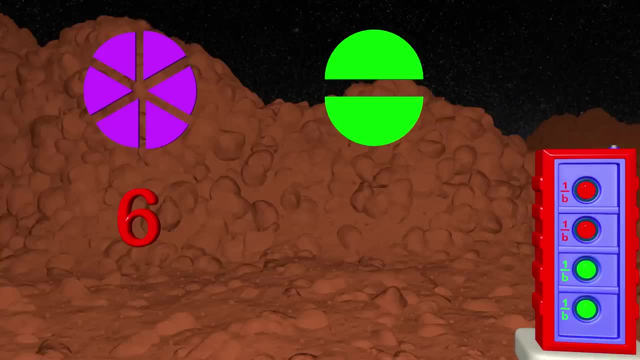 There are 6 equal parts to this circle, so the fraction we want is just one part of the 6 pieces. This fraction is 1 over 6, also called 1 sixth. Now let's look at the circle on the right. 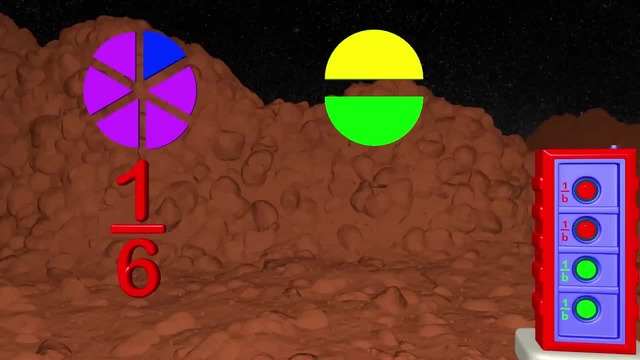 What is the fraction for just one piece of this circle? The fraction is 1 over 2, also called 1 half. The part we need is 1 half of the entire circle. Great job, guys. I am on my way home now. 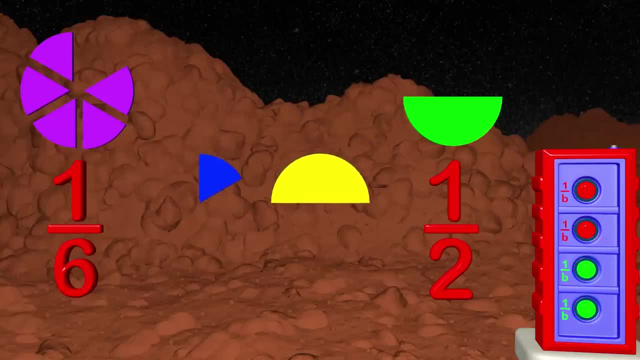 But wait, I noticed something. On the left we have 1 sixth and on the right we have 1 half, but they are definitely different in size. It looks like you get more with 1 half than 1 sixth. This is good to know. 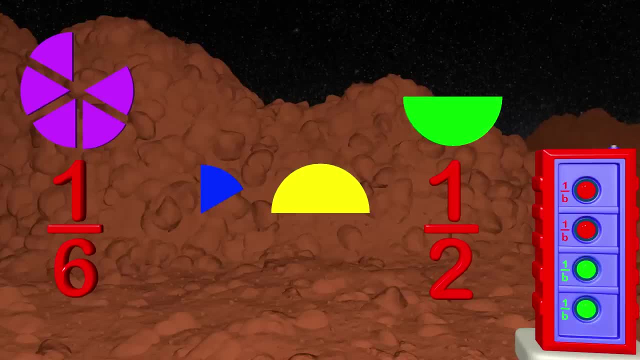 As the denominator or number on the bottom gets bigger, the actual piece itself gets smaller. It is like sharing a pizza: When you eat it with one friend, you both get more than if you share it with 6 friends. Awesome job, my spaceship is now fully charged. 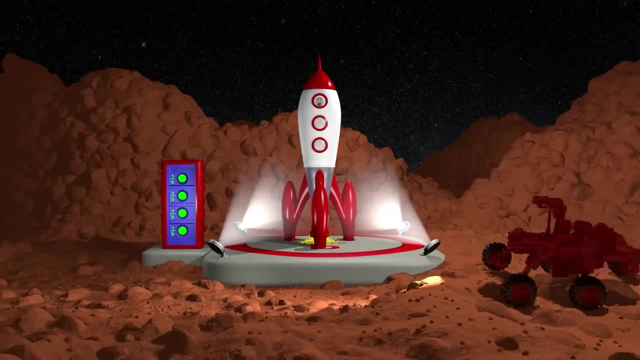 Thanks for helping me charge the batteries with unit fractions. We will see you next time. Goodbye. 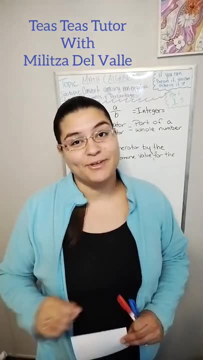 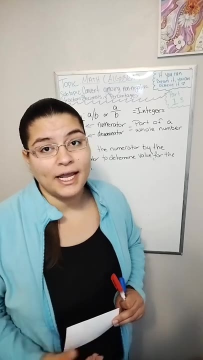 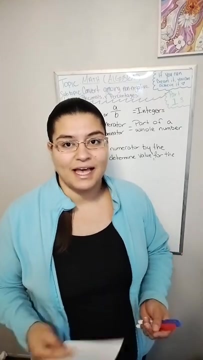 Good morning, welcome back to your TEAS test tutor. I'm your tutor, Melissa del Valle, and today we're going to be in the area of math. Math is a very strong component and, from what I'm gathering, it's getting. it's one of the hardest portions, besides science, to pass the TEAS test. 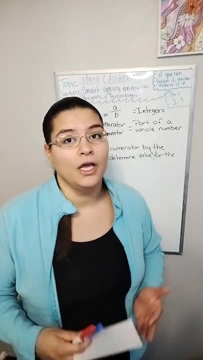 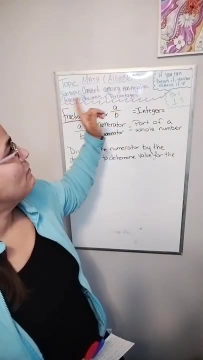 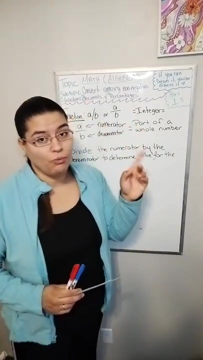 So it's very important to study your math, your algebra, your geometry in order to be able to take the TEAS test. Today we're going to be in algebra between, and the subtopic is going to be converting among non-negative fractions, decimals and percentages. So this is a part one of three. 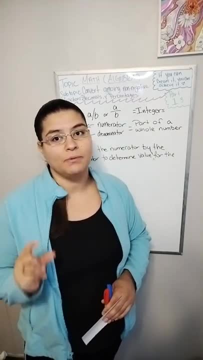 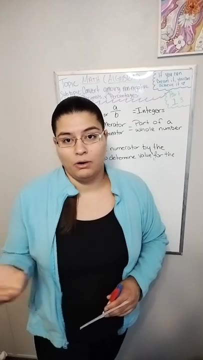 series: I want to take it slow, sweet and simple. The videos: I want to keep them small so that way it could be easily digestible. You can hear them while you're on the go, or several videos in one sitting, However you want to do it. however you want to study. 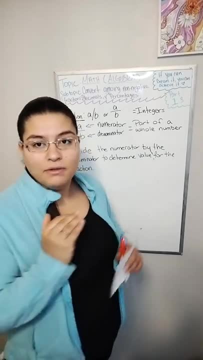 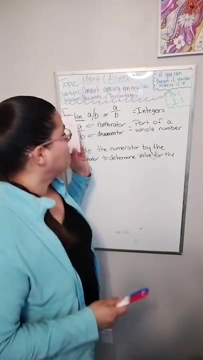 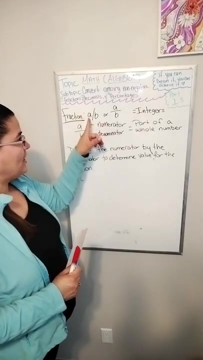 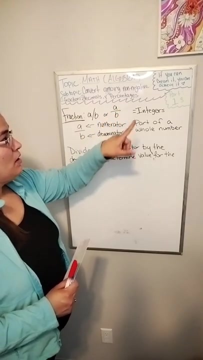 that's up to you. However, studying for studying: this is very important for the TEAS test. Okay, so, uh, fractions, um, you can see from there, right? okay, fractions is anything that, like. it looks like this: you're either going to see it a slash b or a on top of b, and this would equal. these are.